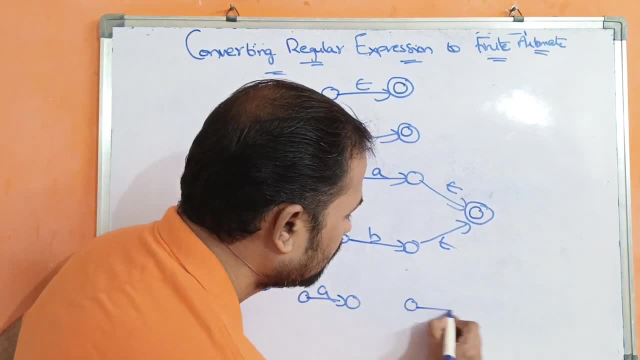 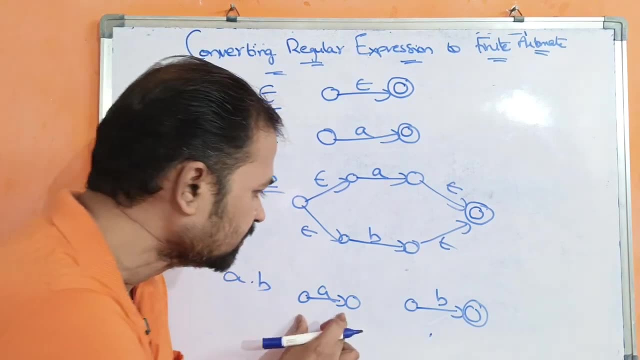 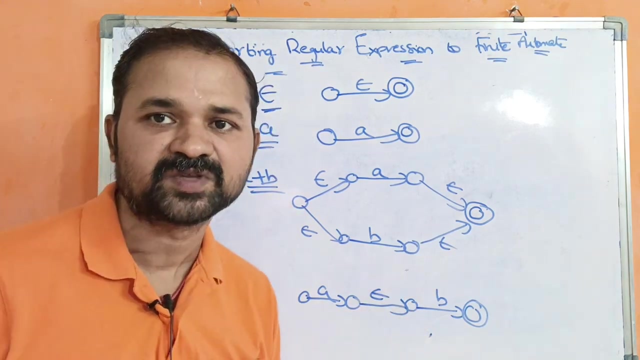 Next, for representing b. also, we can require two states. Let it be the final state. Next, here we can perform concatenation operation between this automata and this automata by applying input a from this state to this state. So like this we can represent a dot b. Let's. 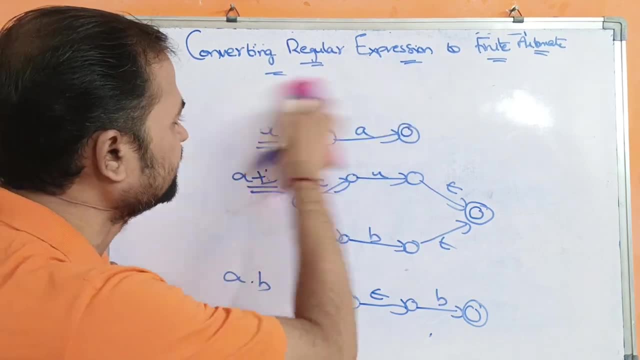 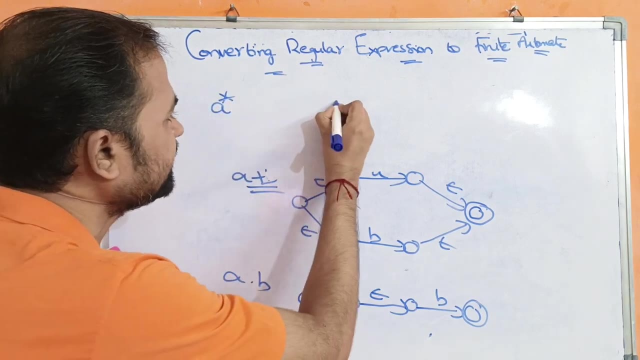 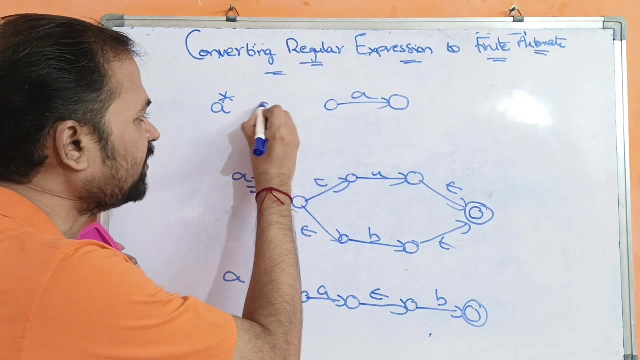 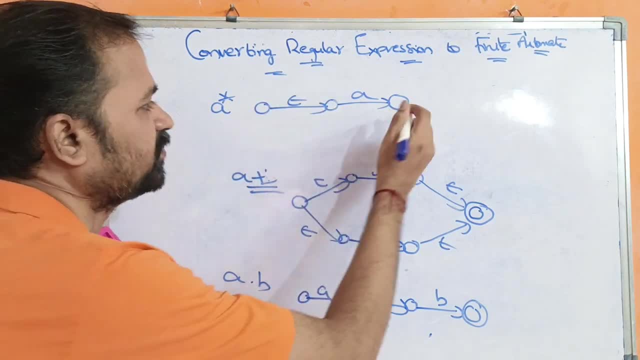 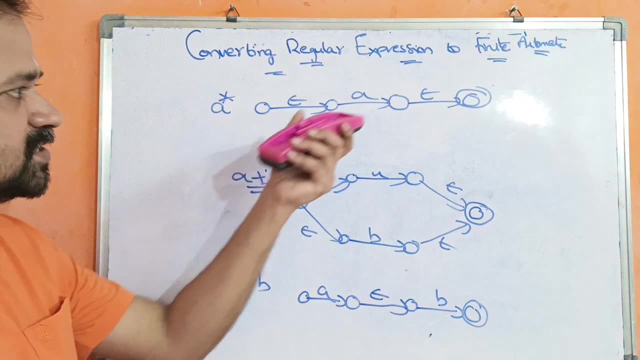 two more states here, and applying epsilon we will move from this state to the new state and applying epsilon we can go from this state to the new state. let it be the final state. So here star means zero occurrences or any number of occurrences, So zero occurrences. 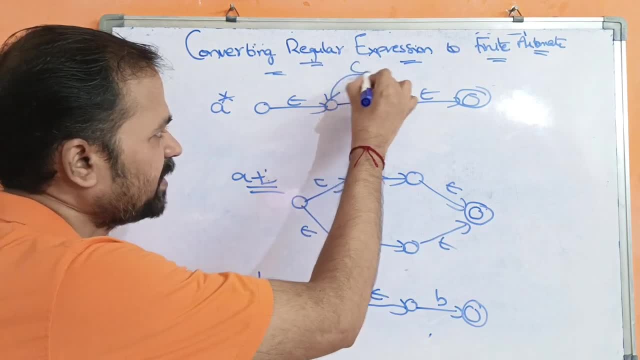 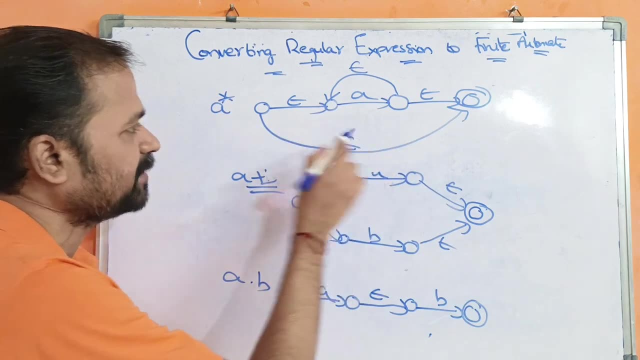 means we have to establish a connection like this and return. So it will be like this: So you can multiply y and y, two people, or just multiply by two people. So y is a. by applying epsilon. next, we can have any number of occurrences, so for that we have to apply epsilon. 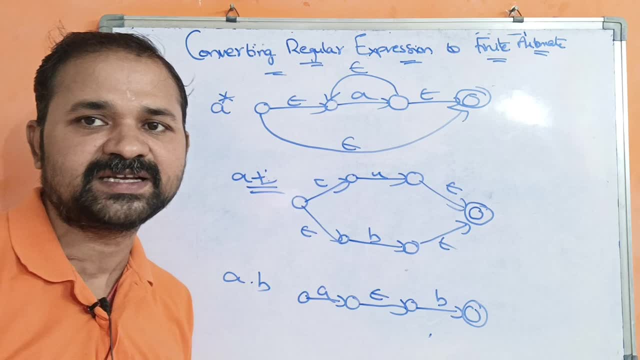 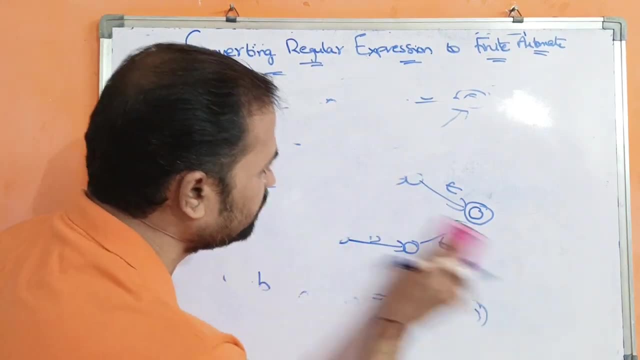 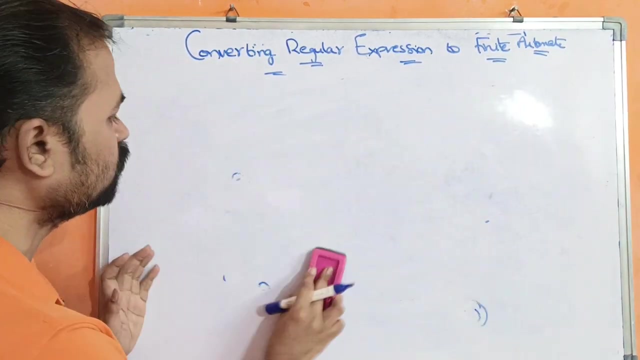 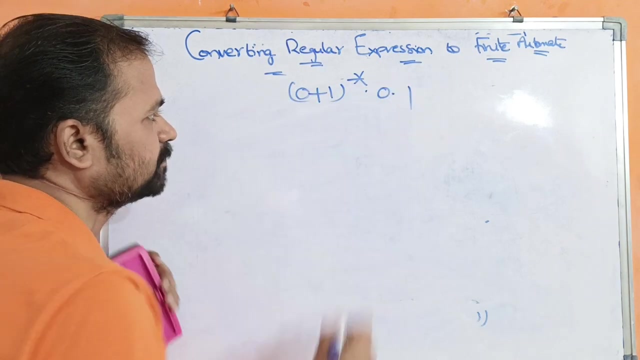 from this state to the final state. so like this we can represent the regular expression. now let us see an example. in order to convert a regular expression into the finite automata, let the regular expression is zero plus one whole star. zero plus one whole star into zero, into one. so first we have to represent zero plus one. 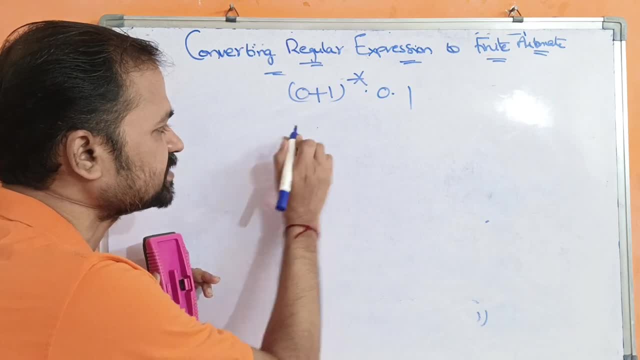 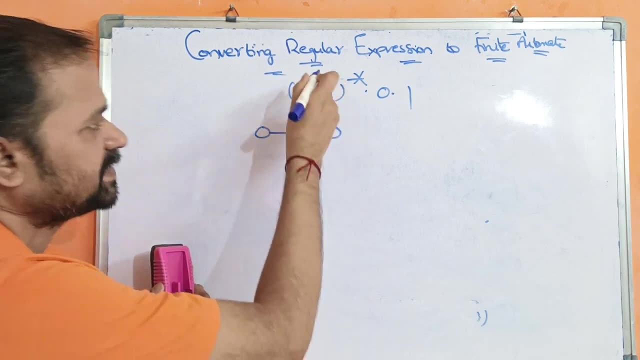 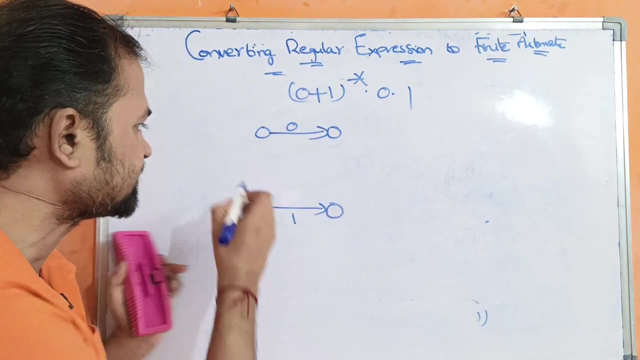 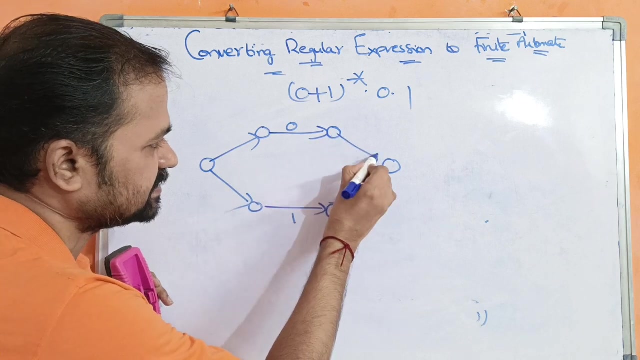 so for representing zero, we require two states. for representing zero, we require two states. next, we can represent one like this. next, plus means we require two more states, we require two more states and we have to represent one like this union operation, so concatenate like this union, like this. so we have to apply epsilon symbol. 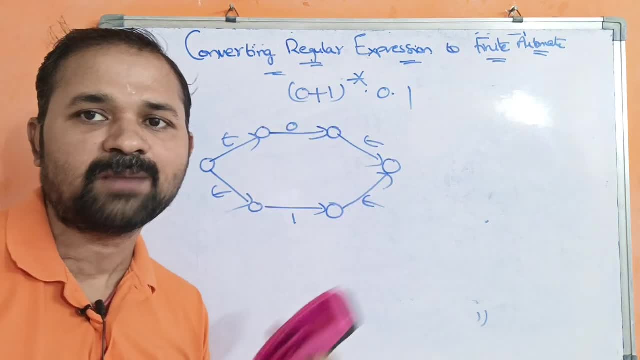 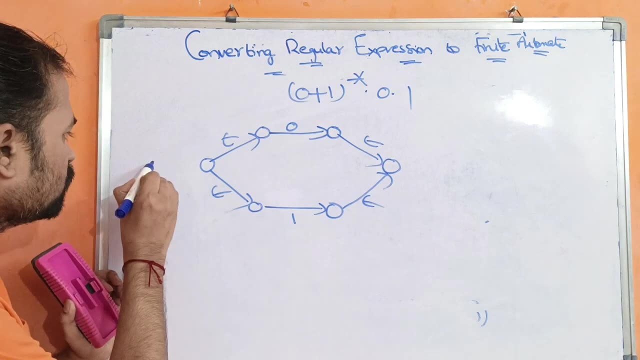 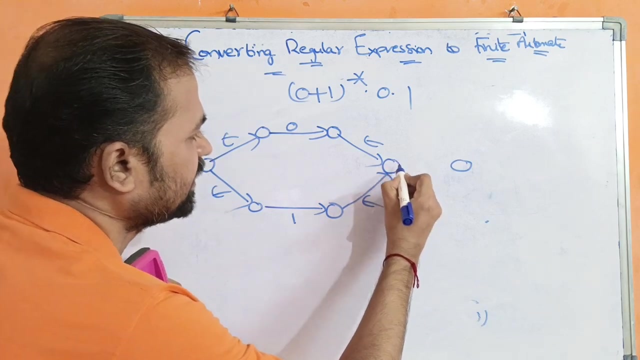 so we can represent zero plus one like this. next we have to apply zero plus one whole star. that is similar to the a star. so in order to have a star, we require two more states. we require two more states. so apply, apply epsilon symbol here. apply epsilon.